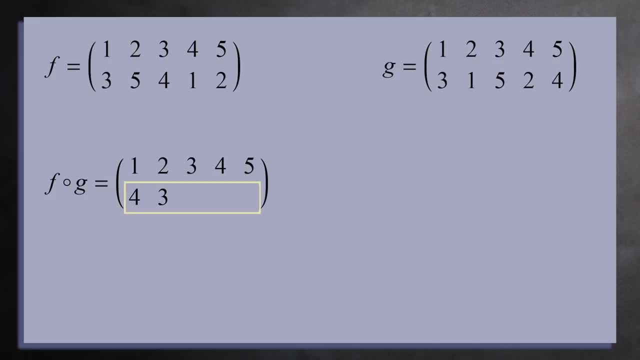 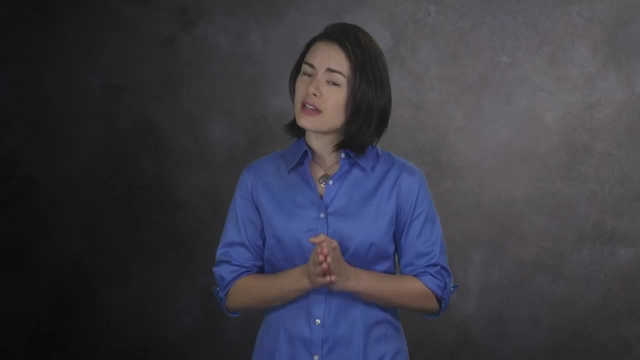 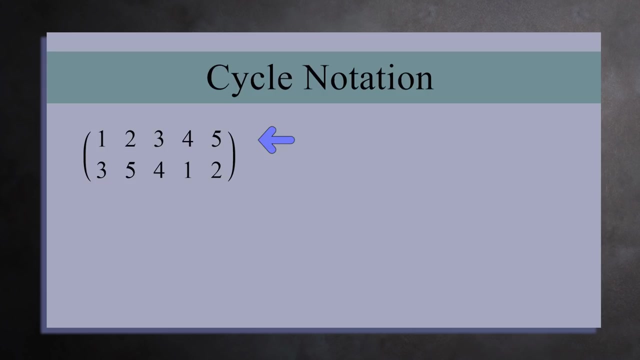 If you do this for the remaining numbers, you get the permutation 4,3,2,5,1. While this way of writing a permutation is clear, it's very time consuming. For each permutation, you have to write every number twice. Cycle notation allows you to write a permutation on a single number. Cycle notation allows you to write a permutation on a single number. Cycle notation allows you to write a permutation on a single number. line, and oftentimes you end up writing fewer than end numbers. Let's now see how to rewrite a permutation using cycle notation. Look at this permutation. Since the top row is always in order, you can read a permutation aloud by only reading the bottom line, 3, 5, 4, 1, 2. 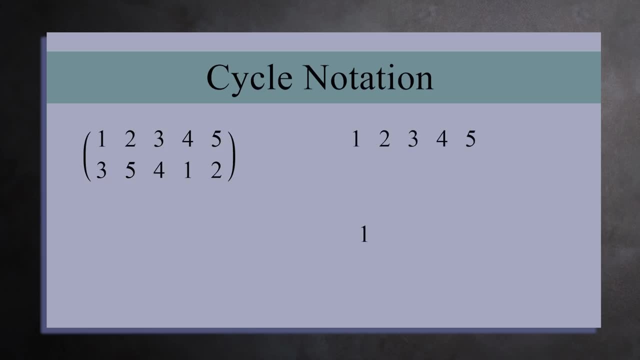 To begin, write down the numbers 1 through 5. We'll start by picking the number 1. Scratch off the number 1 from our list. The rule is to scratch out a number the moment it appears in a mapping. In this permutation, 1 goes to 3, so we can write an arrow showing that 1 maps to 3. You can now scratch out the number 3. Next, 3 goes to 4, so write an arrow showing 3 maps to 4, and then scratch out 4 from our list. And finally, 4 maps back to 1. You describe these mappings in cycle notation by leaving out the arrows and writing 134 inside parentheses. But in your mind, be sure you interpret this as saying 1 maps to 3, 3 maps to 4, and 4 maps back to 1. There are still some numbers in our list, so we're not done yet. 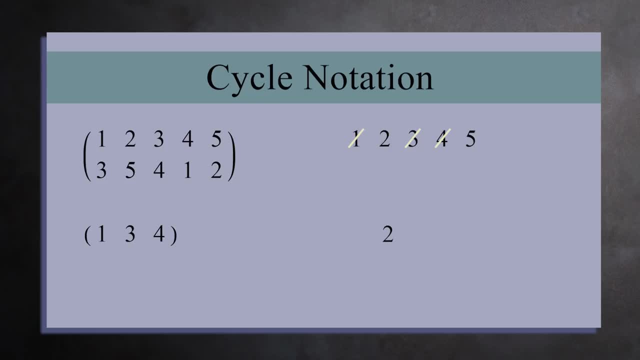 The next number that is not scratched out is 2, so write down 2 and mark it off from our list. 2 maps to 5, so write an arrow mapping 2 to 5, and then scratch out 5. And 5 maps back to 2, so it wraps around. If you leave out the arrows, you get the cycle 2, 5. At this point, there are no other numbers in our list. Thank you for watching! 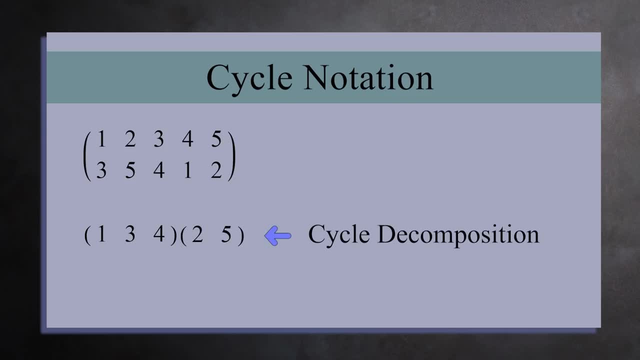 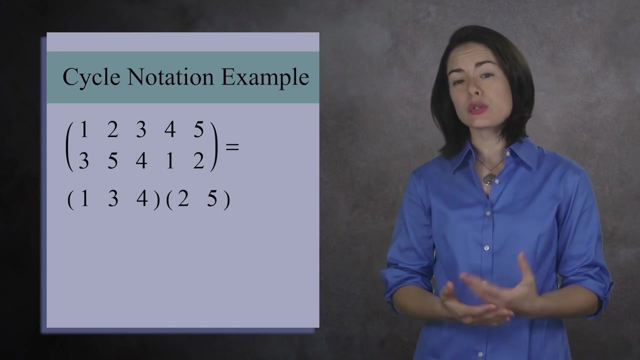 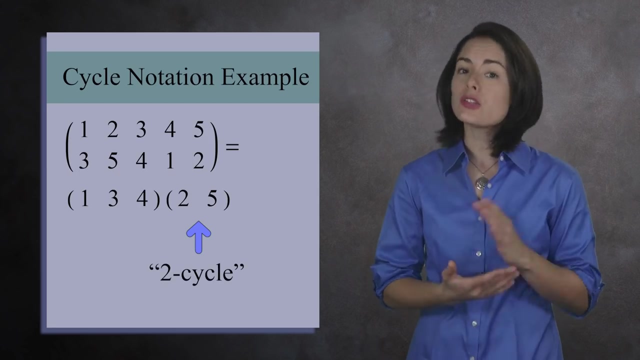 The cycle decomposition of the permutation is 1, 3, 4 times 2, 5. Every number appears in exactly one cycle, and each cycle describes part of the permutation. So the permutation 3, 5, 4, 1, 2 can be written as a product of two cycles. The first cycle has length 3, so we call it a three cycle. The next cycle has length 2, so we call it a two cycle. A cycle of length 2 is also called a transposition. 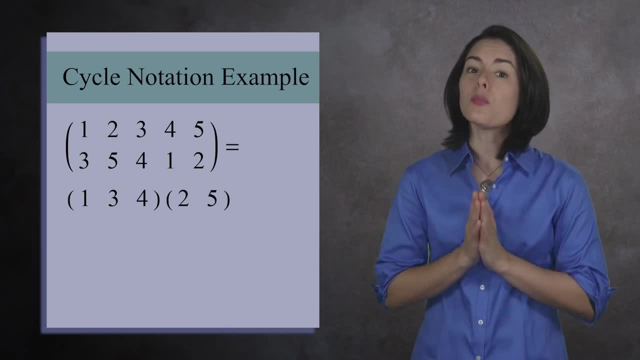 As you can see, cycle notation is much easier to write. But there are more things to learn about cycles, so let's see another example. 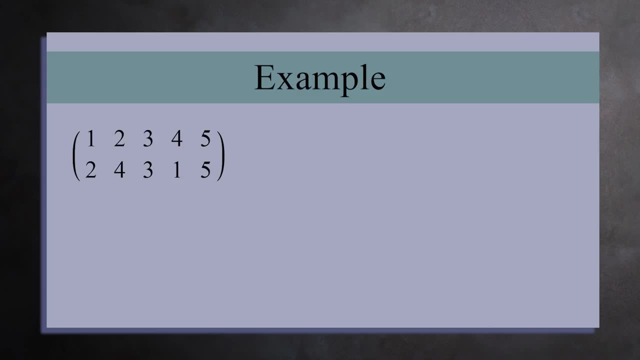 Look at the permutation 2, 4, 3, 1, 5. In the first example, we wrote the numbers 1 through 5, and then started with 1, but there's no reason to start with 1. You can start with any number you want. Let's start with 2. 2 maps to 4, 4 maps to 1, and 1 maps back to 2. This gives us a cycle 2, 4, 1. This is also an analysis of the permutations, so let's look at another example. The permutation 2, 4, 3, 1, 5. Each number is written as a side number, so let's start with 2. The permutation 2, 4, 3, 1, 2. Each number is written as a side This gives us a cycle 2, 4, 1. 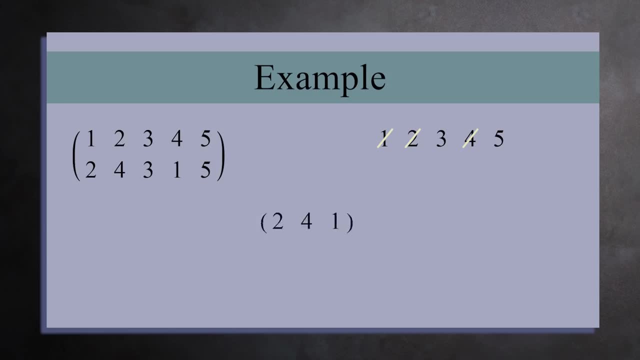 We can mark off these three numbers from our list. Next, we pick another number that has not yet appeared in the cycle and repeat the process. Let's pick 3. 3 maps to itself, so this gives us a cycle with a single number. Scratch off 3. And 5 maps to itself as well. This gives us another cycle with a single number. We can scratch off 5. So this permutation is a product of three cycles. 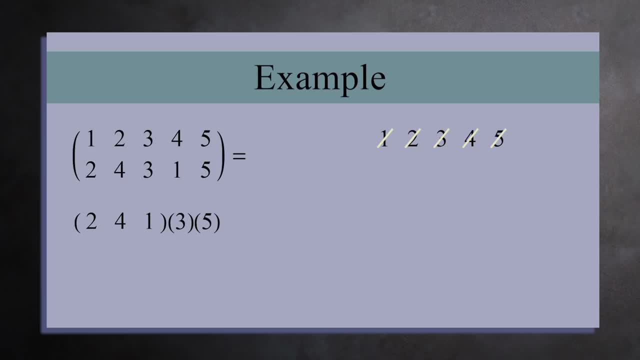 A 3 cycle, a 1 cycle, and another 1 cycle. Here's another shortcut. 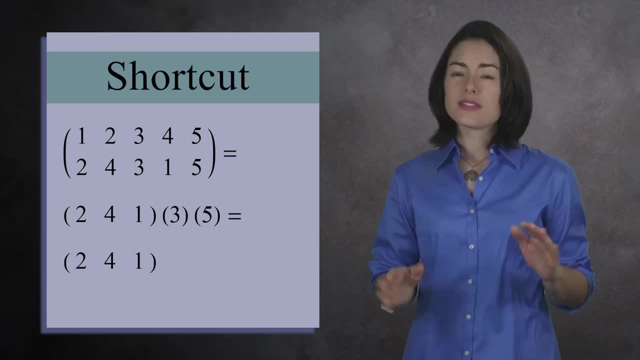 Whenever you have a 1 cycle, you can go ahead and leave it out. This is because 1 cycles do not change any number, so we can safely ignore them. This means the permutation can be written simply as a 3 cycle 2, 4, 1. 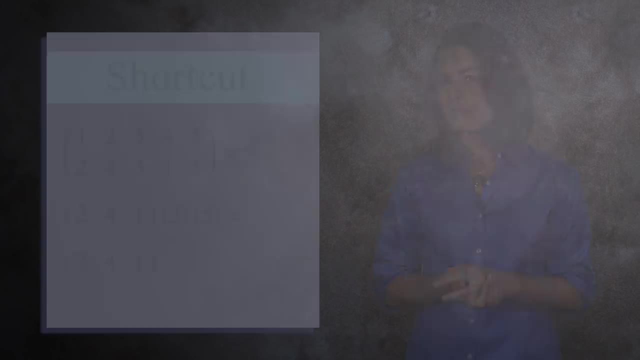 But what if we had started with 4 instead of 2? 4 maps to 1. 1 maps to 2. And 2 maps back to 4. So this gives us a cycle 4, 1, 2. And as before, 3 maps to 3. And 5 maps to 5. And we leave out the 1 cycles. And for completeness, what if you had started with 1? 1 maps to 2. 2 maps to 4. And 4 maps back to 1. Giving us the cycle 1, 2, 4. 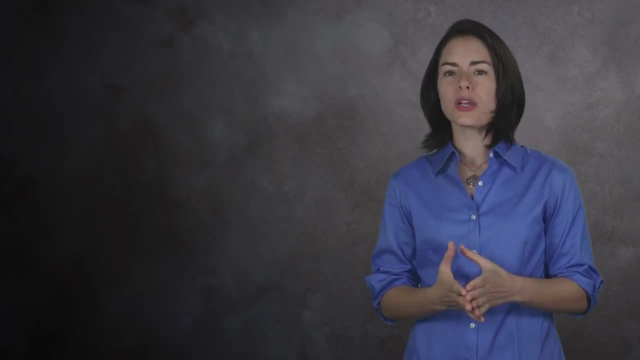 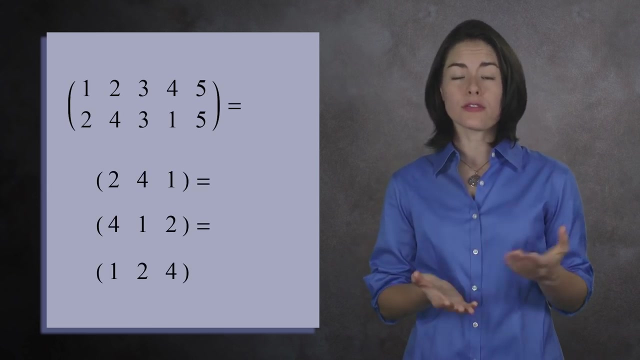 This is curious. It seems you get different answers depending on which number you start with. In the last example, we got three different answers. 2, 4, 1. 4, 1, 2. And 1, 2, 4. But these cycles are all the same. In each cycle, 1 maps to 2. 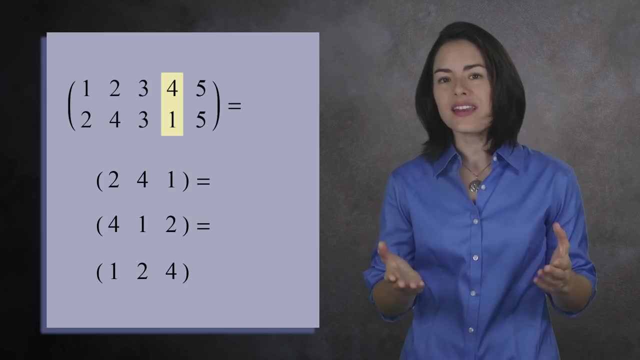 2 maps to 4. And 4 maps to 1. We're just writing the mappings in different orders. 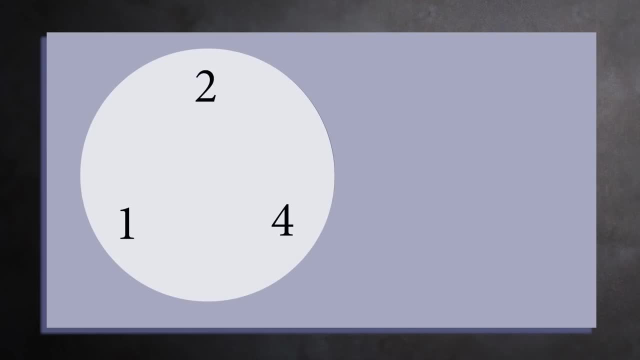 Here's how to visualize what's going on. Imagine these numbers are on a circle, with arrows going clockwise. We then see that 2 maps to 4. 4 maps to 1. And 1 maps to 2. If we start at the top, this gives us a cycle 2, 4, 1. Look what happens if we 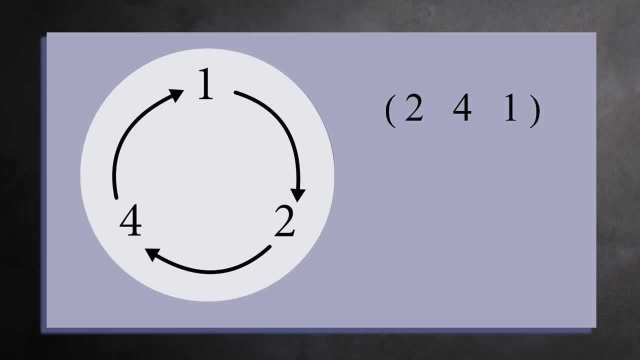 rotate this circle a third of a turn. Then we get the cycle 1, 2, 4. And if we rotate another third, we get the cycle 4, 1, 2. This is why they're called cycles. While we write the numbers in a row, in reality they represent a loop of mappings. These three cycles all represent the same information. A good rule of thumb is to pick the cycle that starts with the smallest number. So in this case, we'd write it as 1, 2, 4. 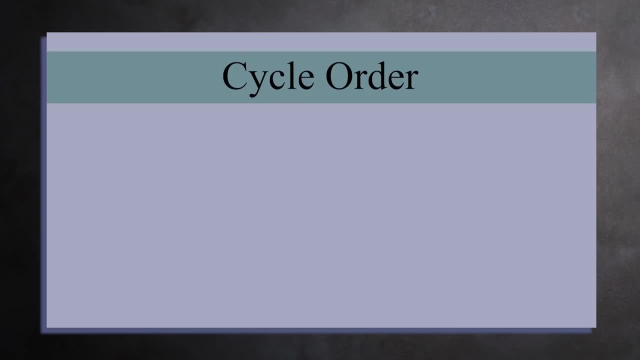 Next, let's talk about the order of the cycles. The cycles in the decomposition. 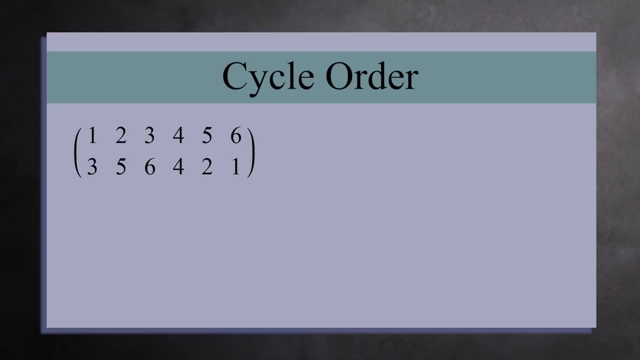 Look at the permutation 3, 5, 6, 4, 2, 1. Let's write this as cycle notation. 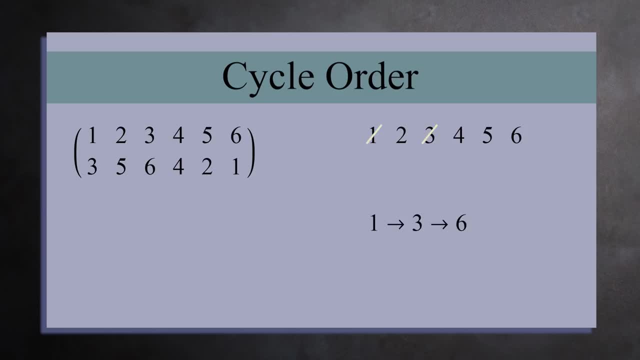 Starting with 1, we see 1 maps to 3, 3 maps to 6, and 6 maps back to 1. This gives us the 3 cycle 1, 3, 6. Notice how I'm checking off the numbers on top once they appear in a cycle. Moving on to the next unchecked number, we see 2 goes to 5, which goes back to 2. This is a cycle 2, 5. 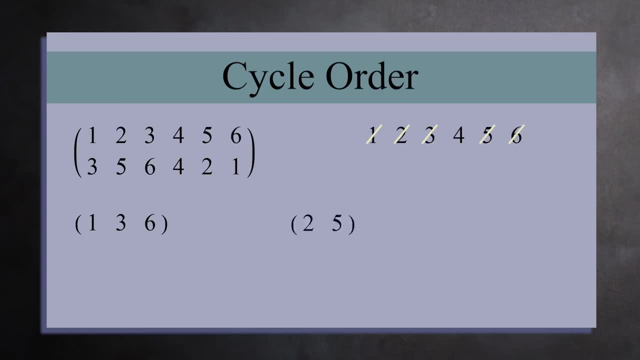 Remember, a 2-cycle is also called a transposition. 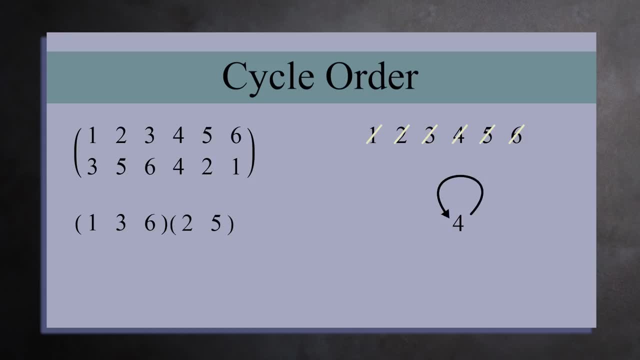 This leaves only 4. 4 goes to itself, so we get the 1-cycle 4. 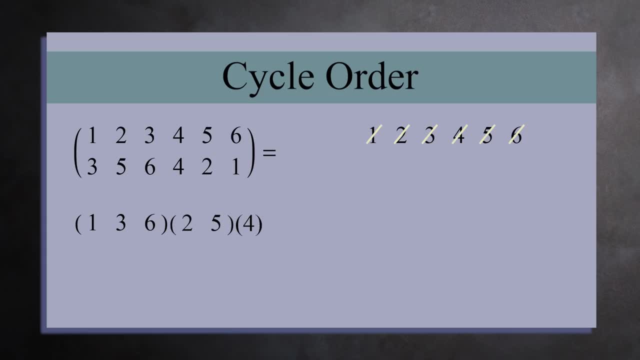 So this permutation can be written as a product of three cycles. 1, 3, 6, 2, 5, and 4. We don't bother writing a 1-cycle, so the permutation is a product of a 3-cycle and a transposition. 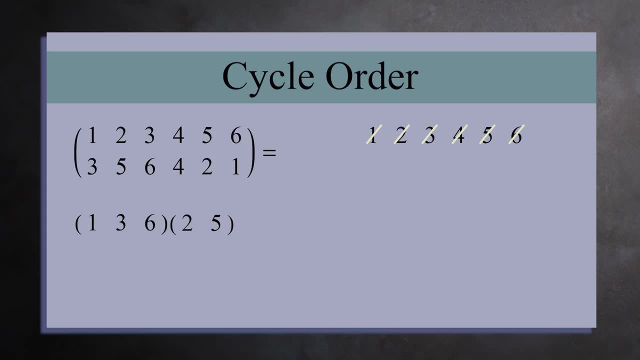 When you write a permutation as a product of cycles, the order of the cycles does not matter. So we could write this permutation as a 3-cycle times a transposition, or as a transposition times a 3-cycle. This is an important point. 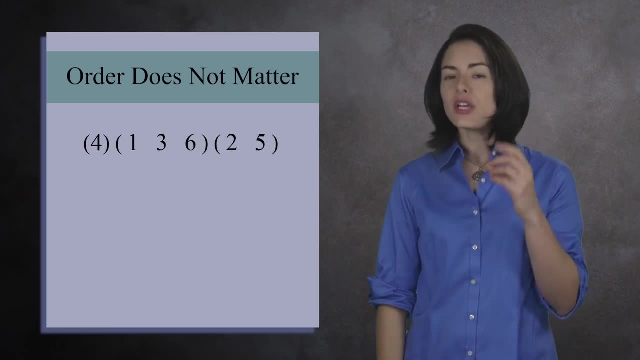 When you decompose a permutation into a product of cycles, the order of the cycles does not matter. But why is this? Here's why. 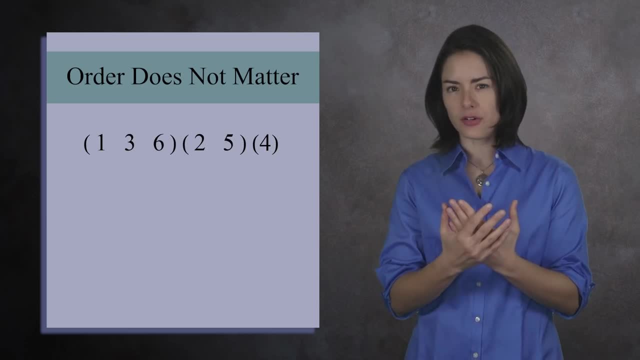 Each cycle can be thought of as a bunch of functions bundled together. And notice that each of the numbers appears in one and only one cycle. So when you plug a number into these functions, it will only be affected by one. It passes through the other cycles unaltered. 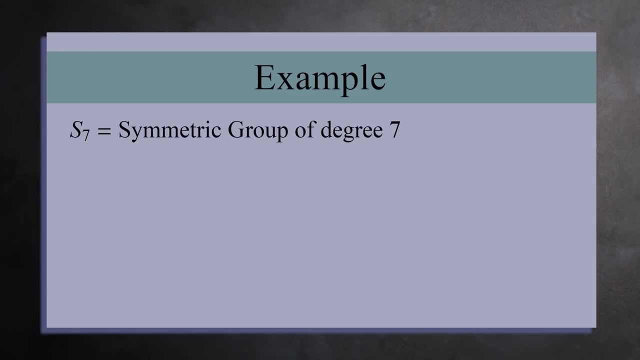 For example, let's look at a permutation from the symmetric group S7. 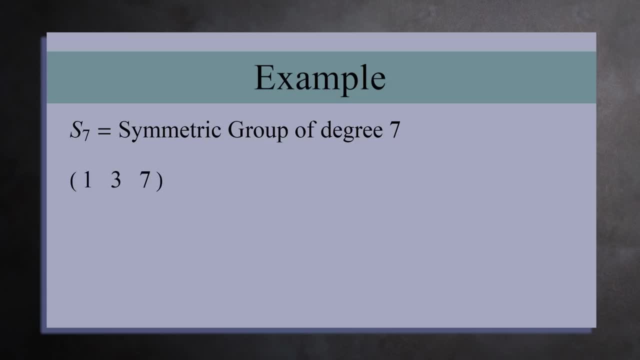 We'll consider the product of the 3-cycle 1, 3, 7 and the transposition 4, 6. 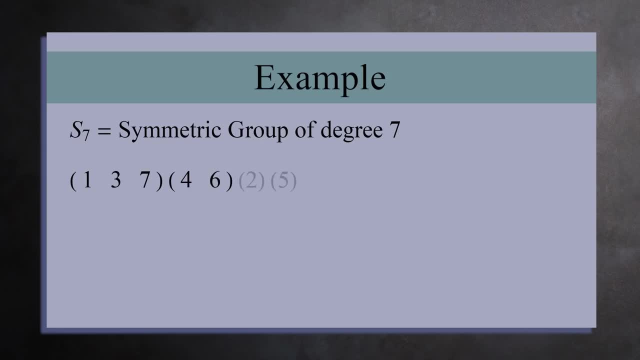 Notice that the numbers 2 and 5 do not appear anywhere. This means they are 1-cycles, and when working with cycles, 1-cycles are invisible. 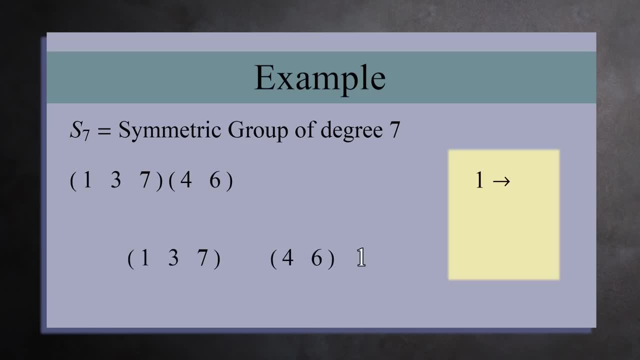 Let's now see what happens to a few numbers. If you plug in 1, it passes through the other cycles unaltered. It passes through the transposition unchanged. Because 1 does not appear in the 2-cycle. When it hits the 3-cycle, 1 is mapped to 3. Next, look at the number 2. 2 is not in either cycle, so it passes through unchanged. 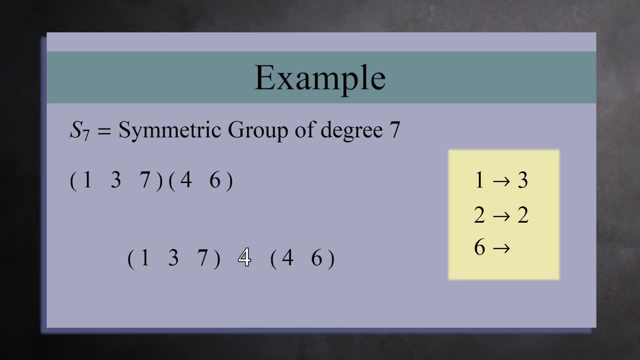 If you plug in 6, the transposition maps it to 4, but the 3-cycle has no effect. The result would be the same if we changed the order of the cycles. And since only one cycle changes any number, the order doesn't really matter. 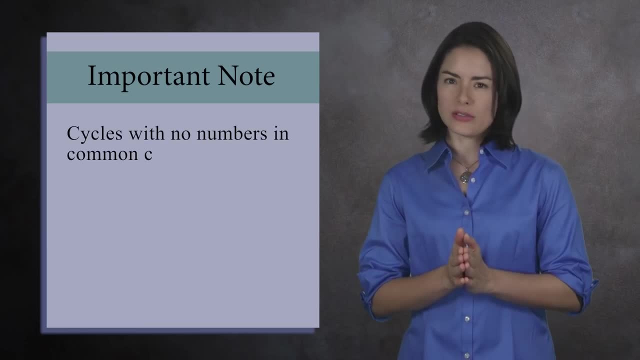 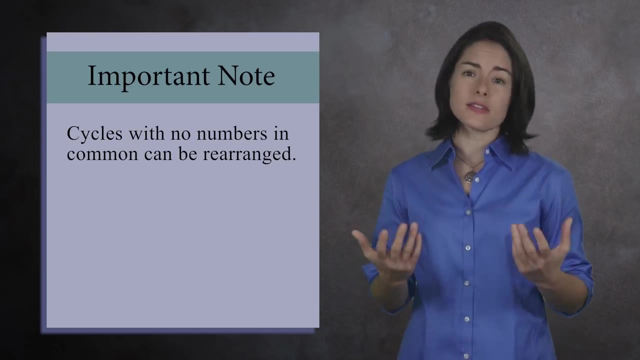 But here's the important part. You can rearrange cycles, but only if no number appears in more than one cycle. When you write a permutation as a product of cycles, this isn't a problem. You're guaranteed each number will only appear in a single cycle. 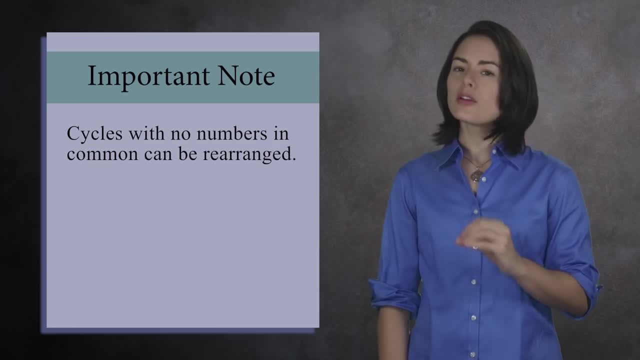 But when you multiply two different permutations, this is no longer the case. 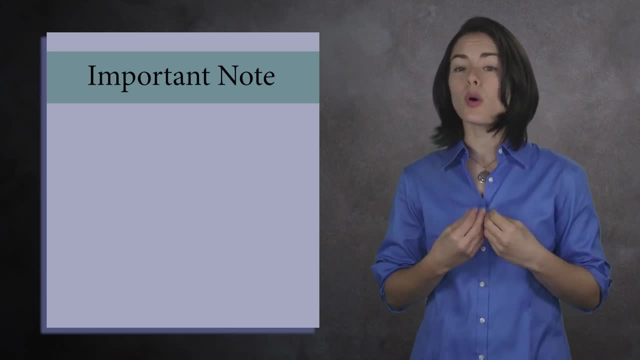 In this situation, you will often find the same number in more than one cycle. So you can't rearrange the cycles. The technical way to say this is as follows. 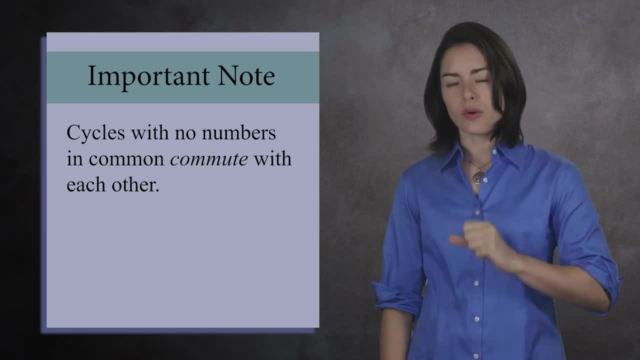 If two cycles have no number in common, then they commute with one another. Let's see an example. 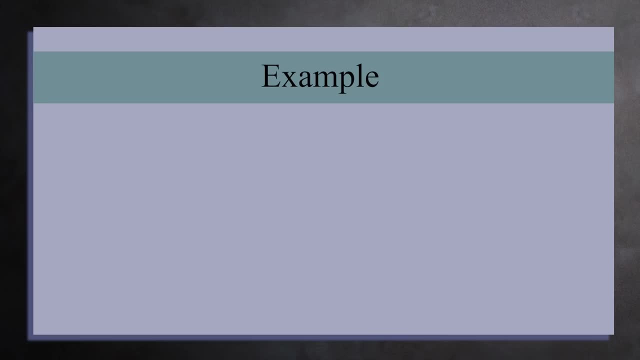 Instead of working with a single permutation, let's multiply two different permutations, A and B. First, let's write these permutations in cycle notation. In A, 1 goes to 3, 3 goes to 2, and 2 goes to 1. 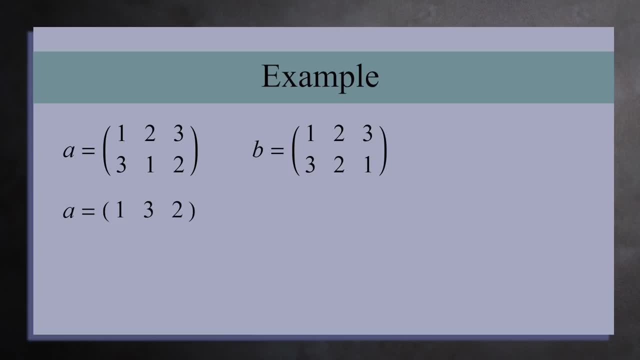 So A can be written as a single 3-cycle, 1, 3, 2. 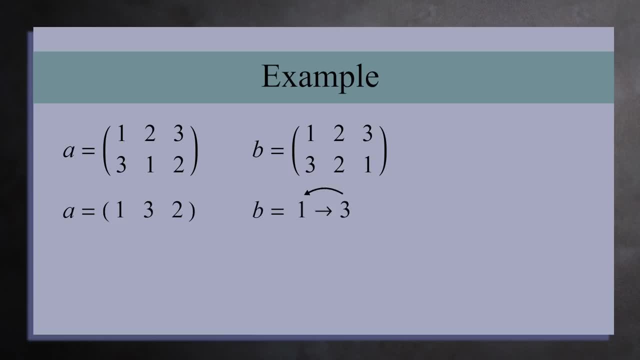 For B, 1 goes to 3, and 3 goes back to 1. And 2 goes to 2. So B is the product of the transposition 1, 3 and the 1-cycle 2. 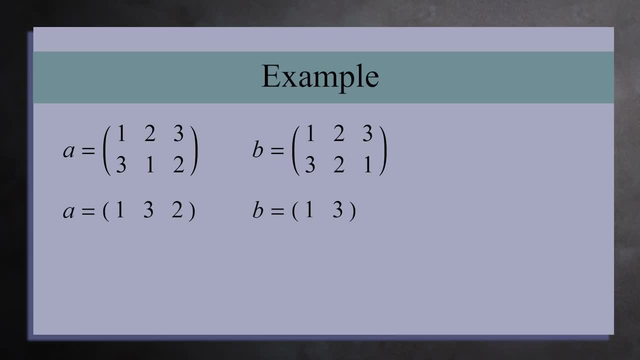 We ignore 1-cycles, so B is simply the 2-cycle 1, 3. 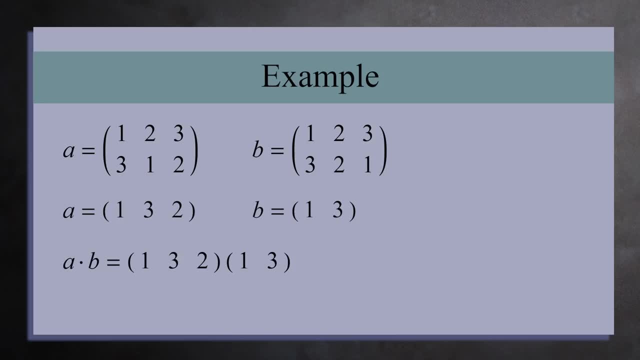 Let's now multiply A and B. Here, the order matters, because the cycles both contain 1 and 3, so they may not commute with each other. 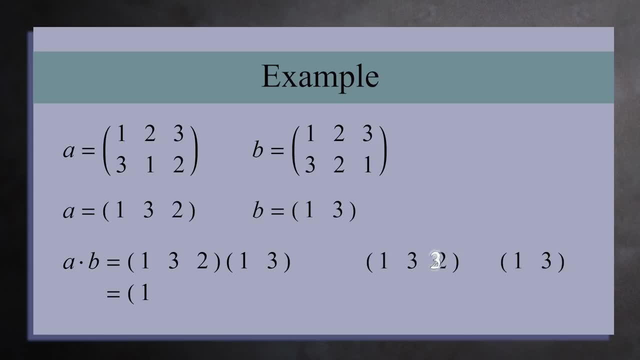 If you plug in 1, the 2-cycle sends it to 3, and the 3-cycle sends 3 to 2. 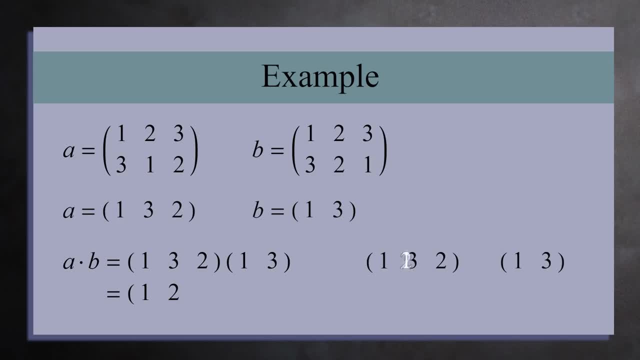 If you plug in 2, the transposition doesn't change it, but the 3-cycle sends it to 1. 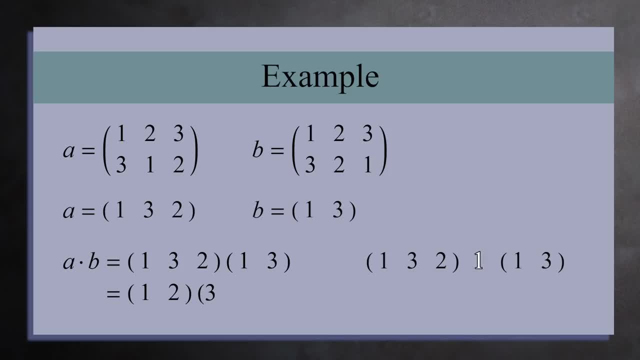 And finally, if you input 3, the 2-cycle sends it to 1, and the 3-cycle then sends 1 to 3, so 3 maps to itself. And we can't ignore 1-cycles. 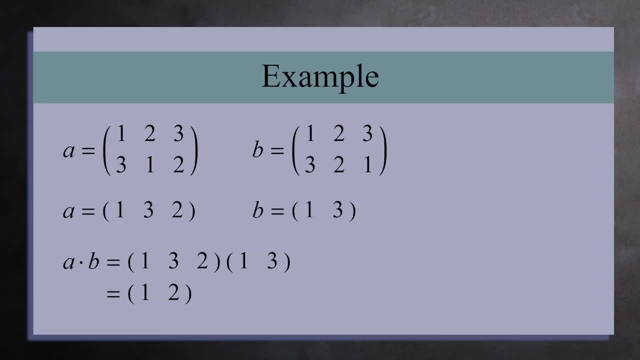 So A times B is a cycle 1, 2. Now look at the reverse, B times A. 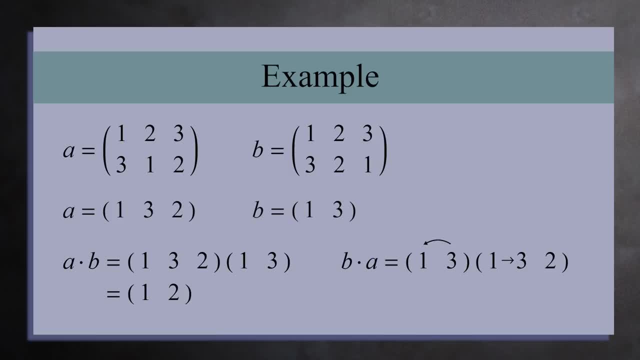 In this case, 1 goes to 3, which then goes to 1. This gives us a 1-cycle. 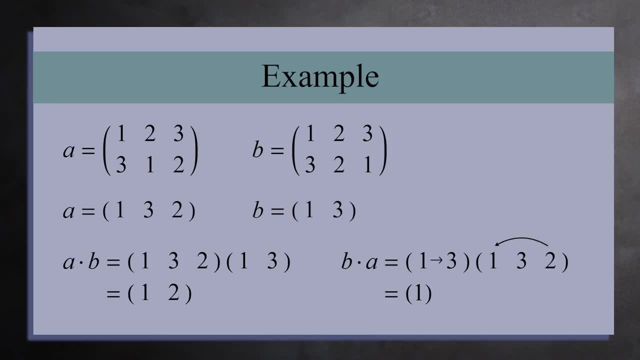 Next, 2 maps to 1, then the transposition sends 1 to 3. If you plug in 3, the first cycle sends it to 2, and the next cycle does nothing to 2. So we're back to where we started, giving us a cycle 2, 3. 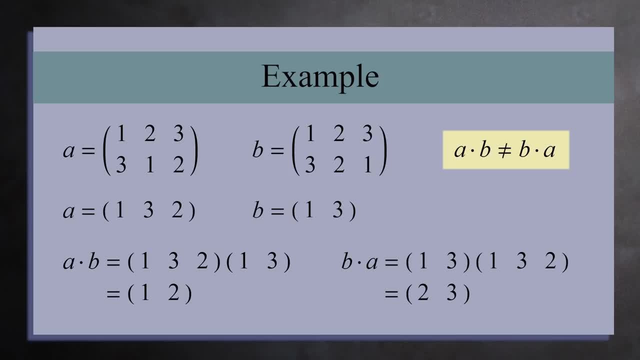 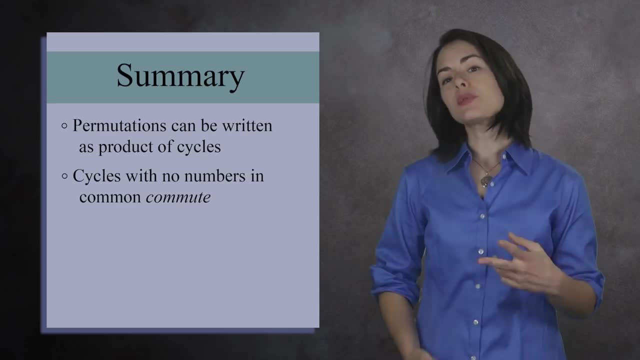 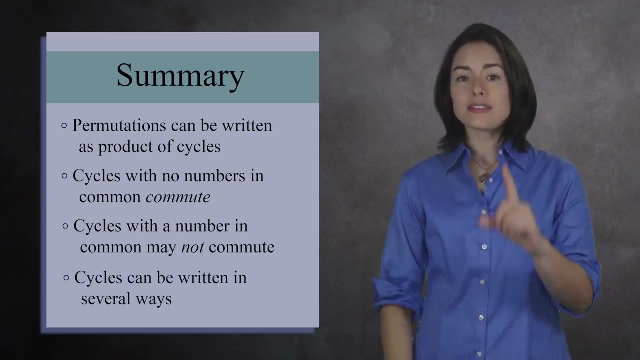 So A times B does not equal B times A. As we've seen, every permutation can be written in the compact cycle notation. If two neighboring cycles have no numbers in common, you can switch them. But if they do share a number, they may not commute. And lastly, any cycle can be written in a number 1. So you can write the cycle in a number of ways, provided the circular order does not change. 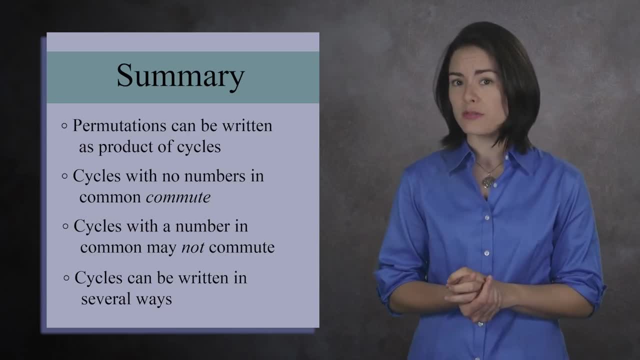 This method of writing permutations is a valuable time-saver when working with symmetric groups.